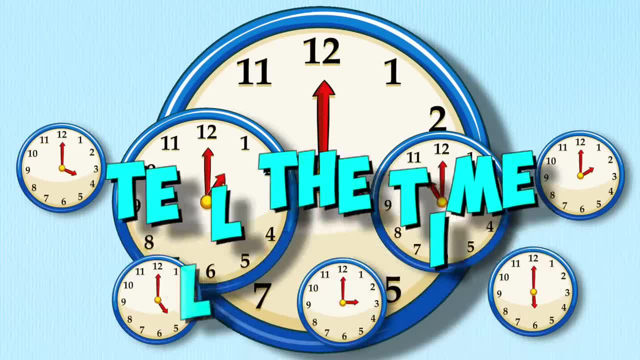 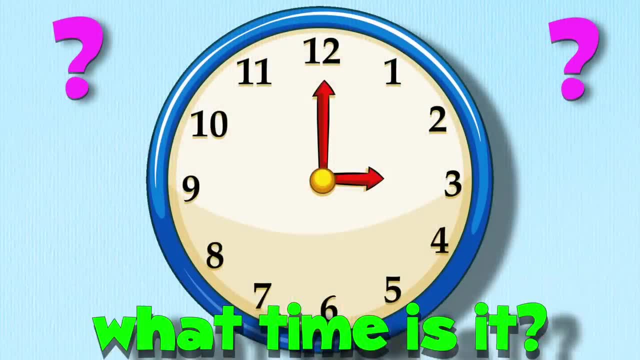 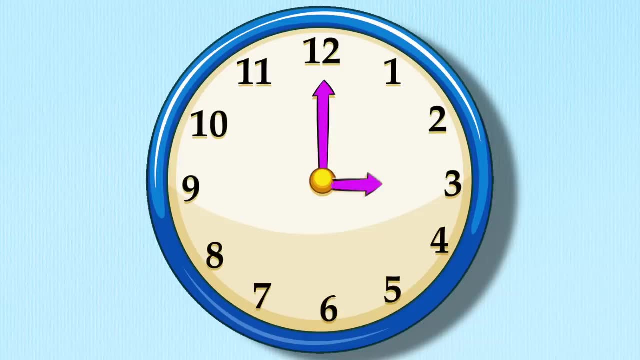 Tell the time, tell the time, tell the time. I can tell time. What time is it? Hmm, I'm not sure What time is it? Wait, I think I know It's three o'clock, Cause the big hand's on the twelve and the small hand's on the three. Is it one o'clock? No, Two o'clock, No, Three o'clock? Yeah, 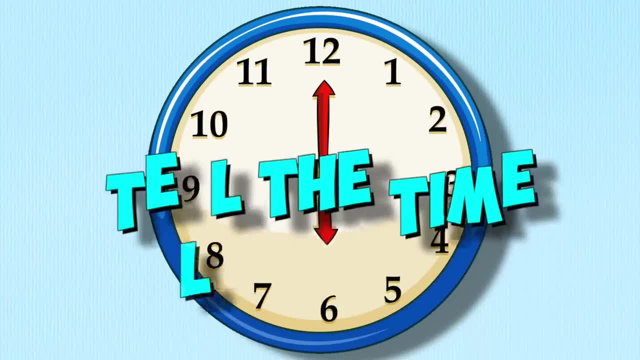 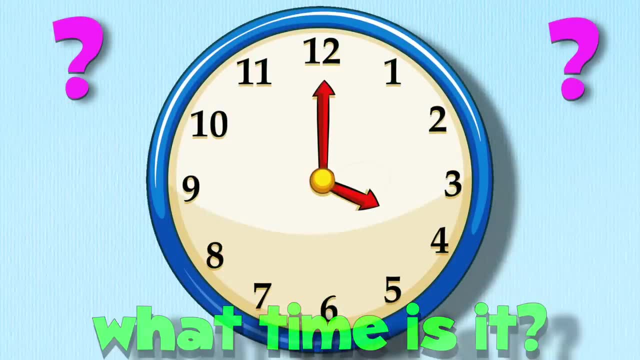 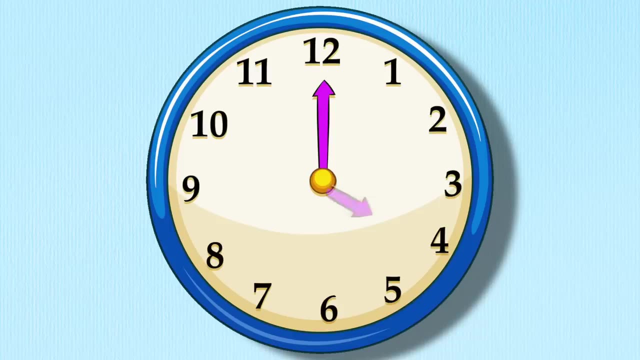 Tell the time, tell the time, tell the time. I can tell time. What time is it? Hmm, I'm not sure. What time is it? Wait, I think I know It's four o'clock, Cause the big hand's on the twelve and the small hand's on the four. Is it two o'clock? No, Three o'clock, No, Four o'clock? Yeah. 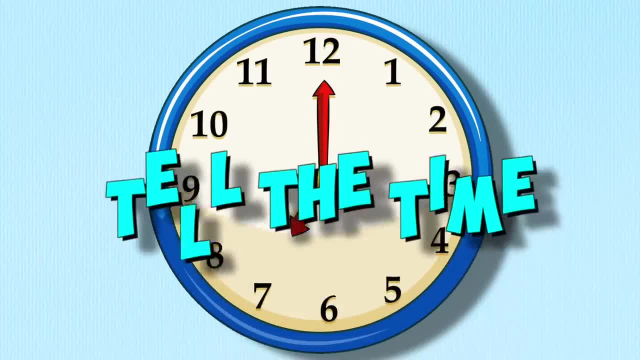 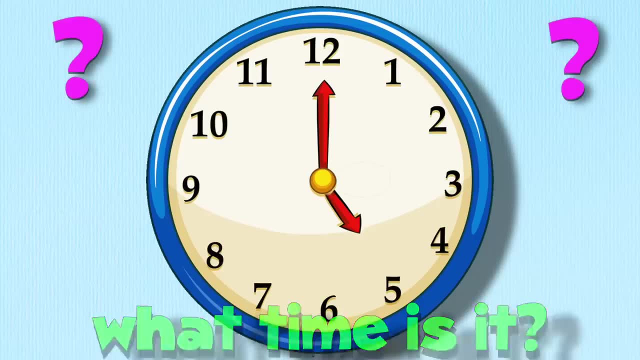 Tell the time, tell the time, tell the time. I can tell time. What time is it? Hmm, I'm not sure. What time is it? Wait, I think I know It's five o'clock, Cause the big hand's on the twelve and the small hand's on the five. 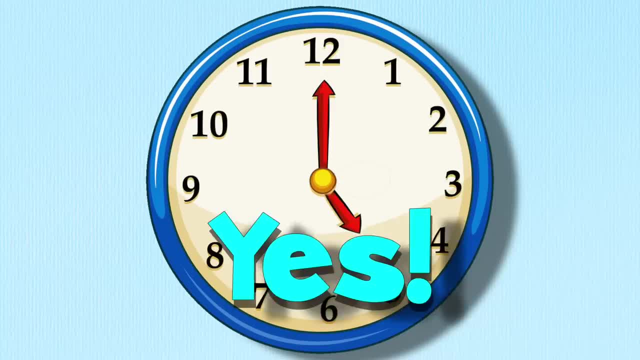 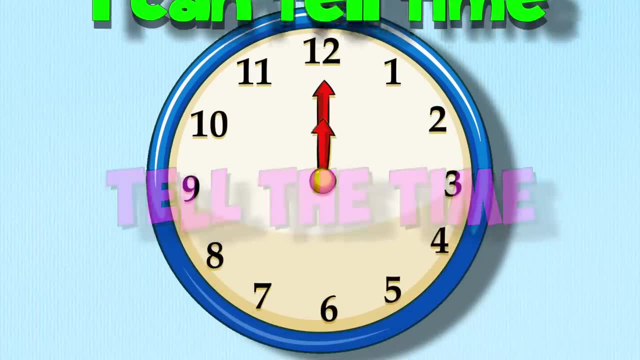 Is it three o'clock, No, Four o'clock, No Five o'clock? Yeah, Tell the time, tell the time, tell the time. I can tell time. What time is it? I'm not sure. What time is it Wait? I think I know. 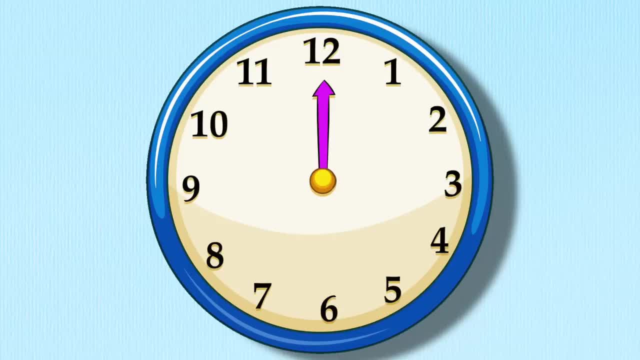 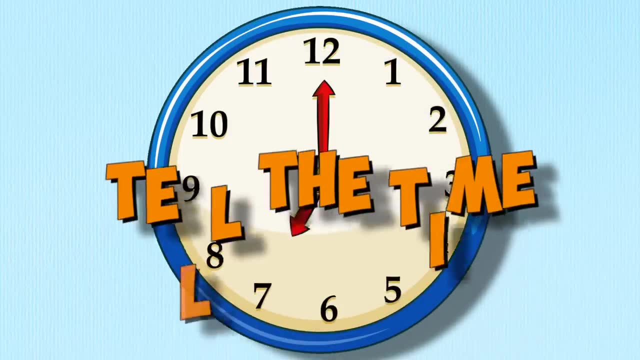 It's six o'clock, Cause the big hand's on the twelve and the small hand's on the six. Is it four o'clock? No, Five o'clock, No, Six o'clock. Yeah, Tell the time, tell the time, tell the time. 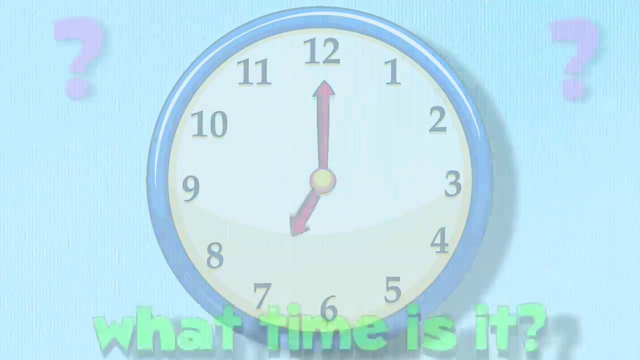 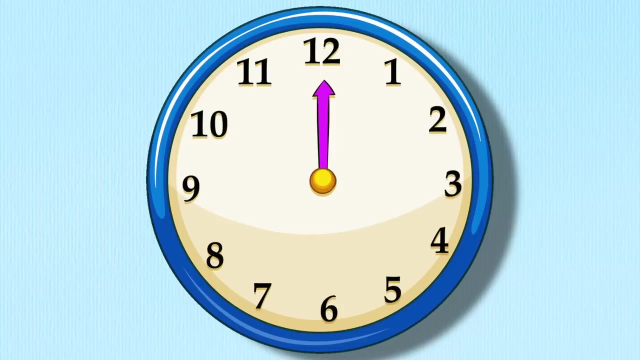 I can tell time. What time is it? I'm not sure. What time is it? Wait, I think I know It's seven o'clock, Cause the big hand's on the twelve and the small hand's on the seven. Is it five o'clock? No, Six o'clock, No, Seven o'clock, Yeah. 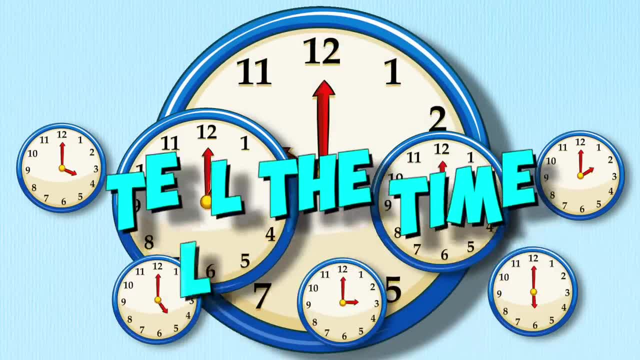 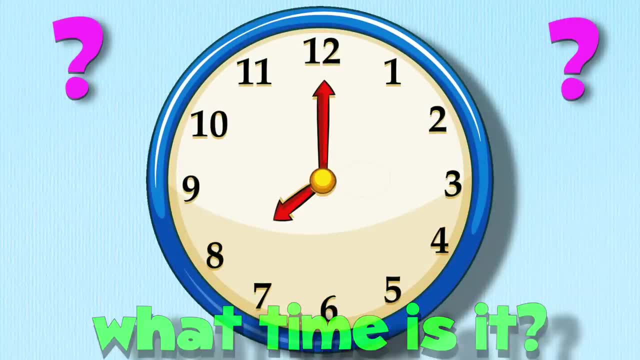 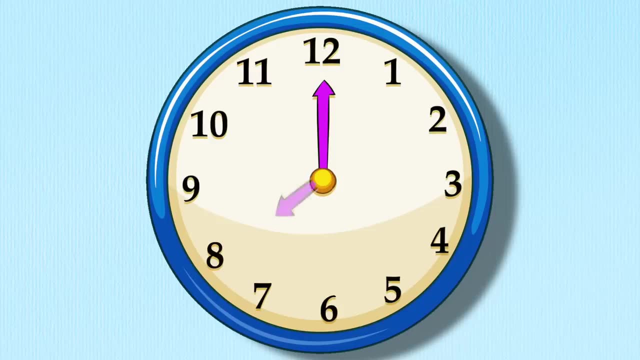 Tell the time, tell the time, tell the time. I can tell time. What time is it? I'm not sure. What time is it? Wait, I think I know It's eight o'clock, Cause the big hand's on the twelve and the small hand's on the eight.